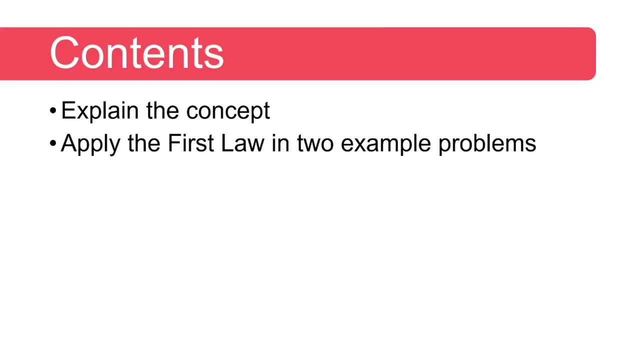 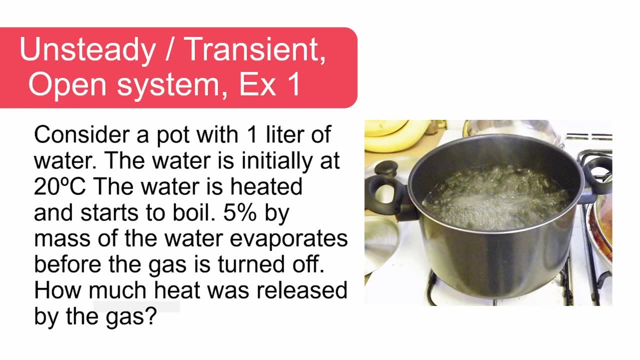 contents for this video. we will explain the concept of transient open systems and apply the first law into example problems. so here is our first example. consider a pot containing one liter of water and the water is initially at 20 degrees celsius. the water is heated and starts to boil. five percent by mass of the water evaporates before the gas is turned. 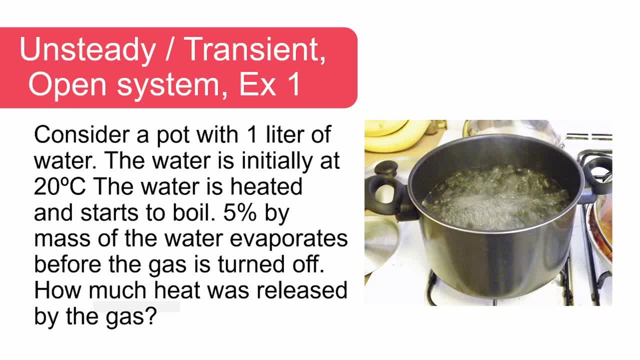 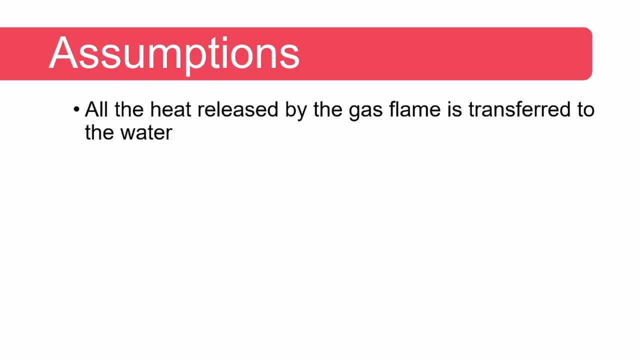 off. the question now is how much heat was released by the gas. first, we need to make some assumptions. we will assume that all the heat released by the gas flame is transferred to the water. the ambient pressure is assumed to be 100 kilopascal. we also assume that one liter of 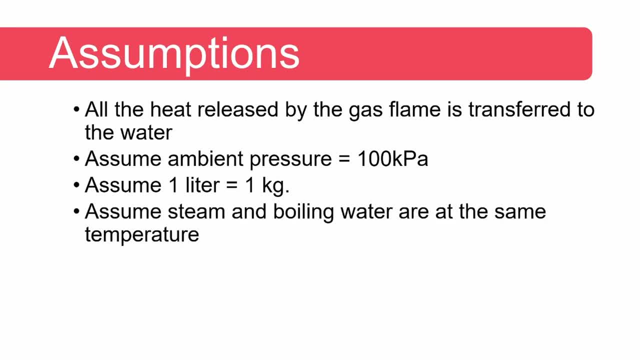 water equals one kilogram. we also assume that the steam is saturated and at the same temperature as the boiling water. the temperature of the pot will also increase from 20 degrees celsius to 100 degrees celsius, but in this example we are going to ignore the heat required to 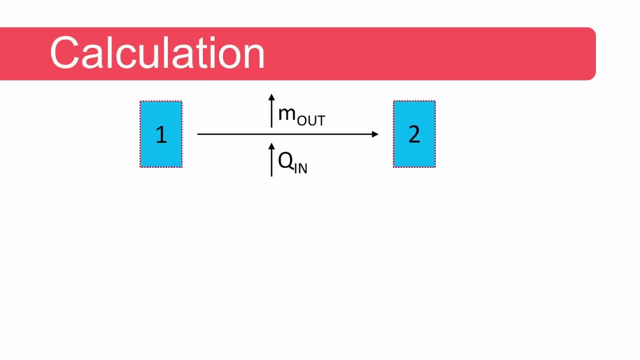 heat up the pot. now let's first draw picture. We consider only the water. The system boundary is given by the red dashed light. Even though the volume of the system will decrease slightly due to the small amount of steam escaping and therefore some boundary work will be done, we assume that the amount 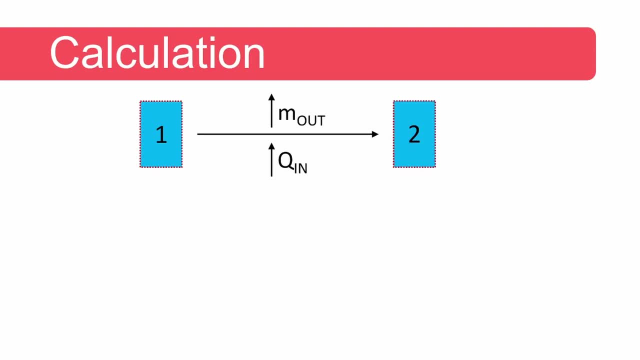 of boundary work is negligibly small. You can calculate its value if you are interested in confirming the validity of our assumption. Now, steam flows across the system boundary and heat is also transferred across the system boundary, as shown in our picture, And the state changes from 1 to 2.. Now let us start our analysis. Energy conservation requires. 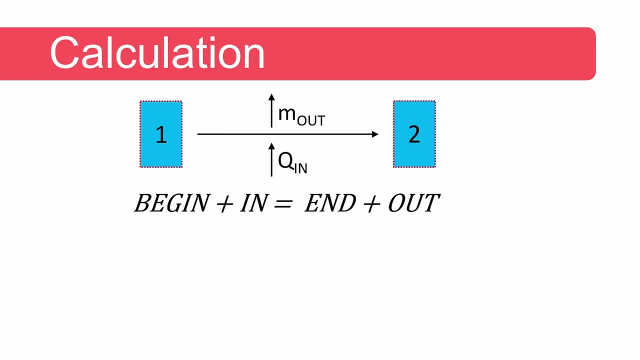 that the energy in the beginning plus the energy that flows into the system is equal to the energy at the end plus the energy that has left the system. The energy in the beginning is equal to the mass of water multiplied by the internal energy of the liquid water, The. 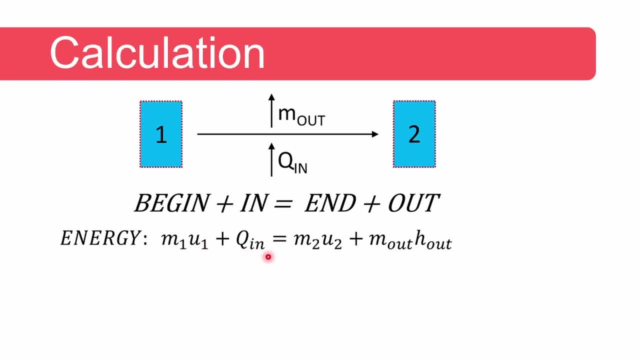 only energy that enters the system is the heat Q. Let us now consider the right hand side of the equation. The energy at the end of the system is equal to the energy that flows into the system. The energy at the end is the mass of liquid water multiplied by the internal energy of. 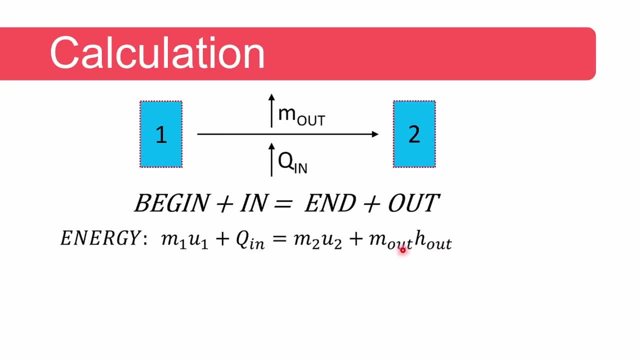 the hot water Energy leaves the system in the form of steam and, as it is flowing, its energy content is given by enthalpy. M1 is the mass of water at the beginning and is given in the problem statement. We can read the value of U1 from the tables: the internal: 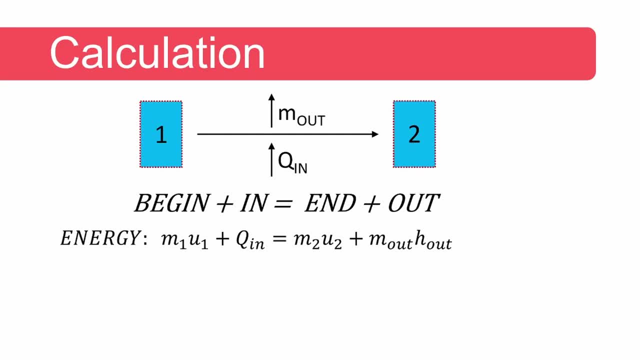 energy of water at 20 degrees Celsius and we want to determine the value of Q. The value of M2 is given in the problem statement and the value of U2 is given in the problem statement. The value of U2 is that of Saturated Liquid Water at 100 kilopascal. We can Calculate M. 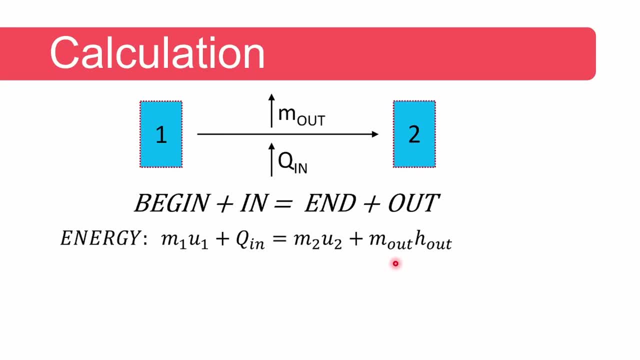 out using the mass conservation which gives the following equation: M1 is given in the problem statement. The value of M1 equals M2 plus M out, which allows us to calculate M out. The value of enthalpy out is that of Saturated Steam at 100 kilopascal. Note that 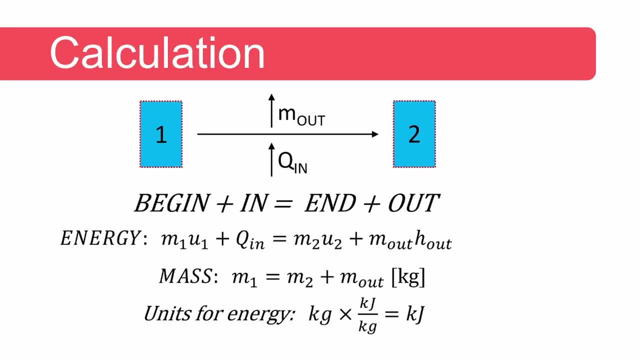 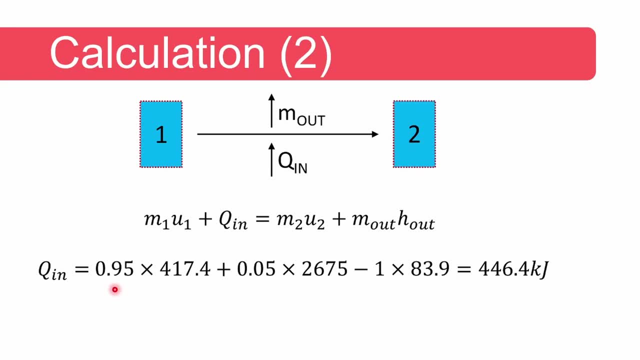 the units for energy is kilogram times kilojoule per kilogram, which is equal to kilojoules. This value of U2 is given in the problem statement. We can rearrange the equation in the PREFERENCE. the equation in the previous slide to calculate Q. Now M2 is equal to 0.95.. Using the steam tables: 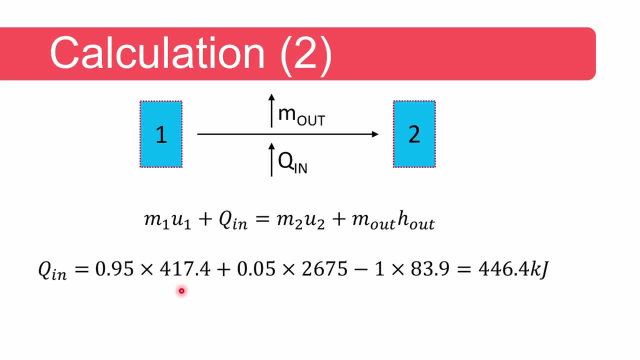 we can determine the internal energy of saturated water at 100 kilopascal, which is 417.4 kilojoules per kilogram M. out is 5% of the initial mass evaporated and the enthalpy is that of saturated steam at 100 kilopascal. The water is initially sub-cooled, but we assume its internal energy is. 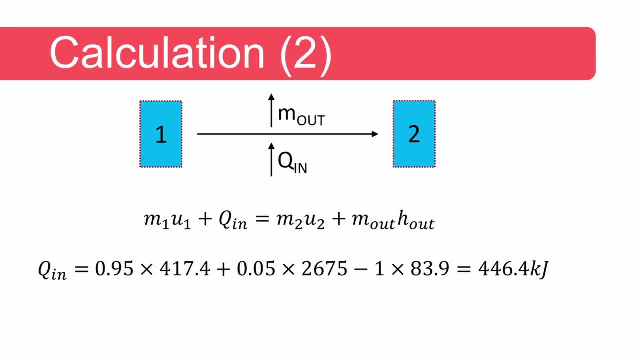 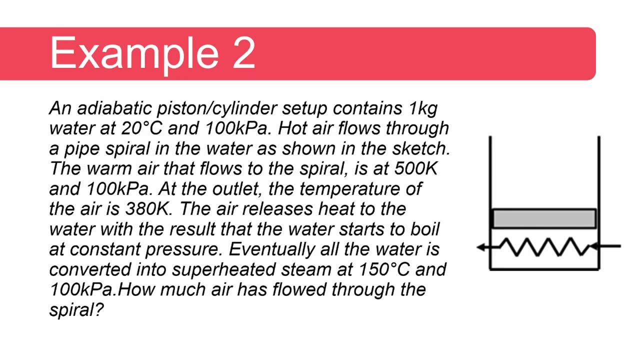 the same as that of saturated liquid water at the same temperature of 20 degrees Celsius. We can now calculate the value of Q and we get a value of 446.4 kilojoules. See if you get the same value as me. Let's consider a second example. Example 2 reads as follows: An adiabatic piston cylinder. 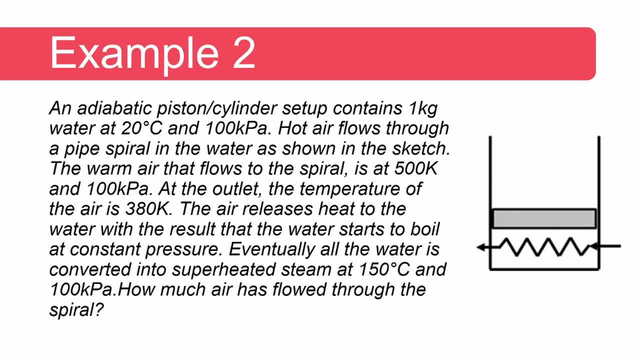 setup contains one kilogram of water at 20 degrees Celsius and 100 kilopascal. Hot air flows through the pipe spiral in the water. as shown in the sketch. The warm air that flows to the spiral is at 500 Kelvin and 100 kilopascal At the outlet, the 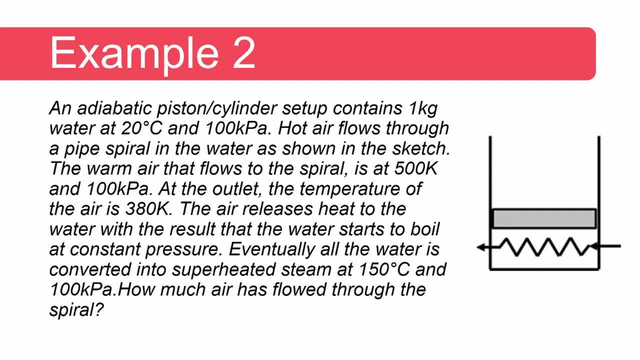 temperature of the air is 380 Kelvin. The air releases heat to the water, with the result that the water starts to boil at constant pressure. Eventually, all the water is converted into superheated steam at 150 degrees Celsius and 100 kilopascal. The question asks how much air has. 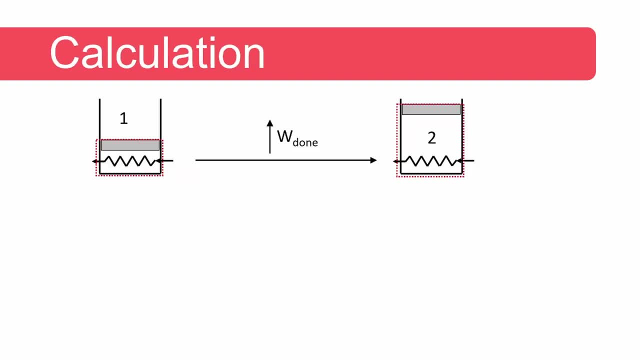 flowed through the spiral to achieve this state. First again, let's draw a picture. The system boundary again is given by the red dashed lines. The volume of the system increases and therefore boundary work is done, pushing away the atmosphere. Air flows in and out of the system. 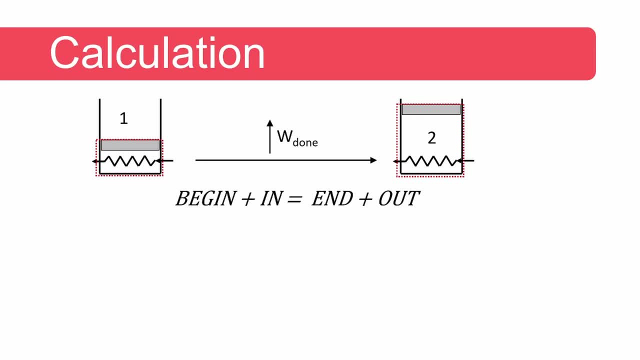 but we assume no air accumulates inside the coil. Conservation of energy means that the energy in the beginning plus energy flowing in equals the energy of the system at the end plus the energy out. In mathematical terms, the energy in the beginning is equal to the mass of water times the. 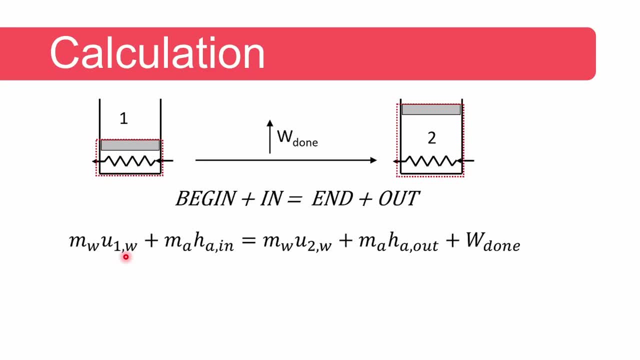 energy of water at state one and the amount of energy associated with the air that flows across the system boundary into the system is the mass of air multiplied by the enthalpy of air at 500 Kelvin. This value can be read from the ideal gas air table On the right hand side of the equation. 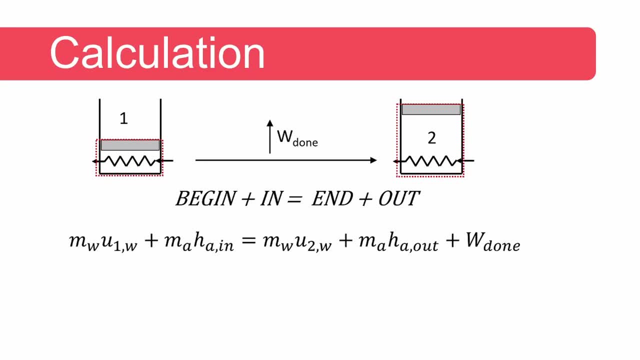 the energy in the system at the end of the process is equal to the mass of superheated steam multiplied by its internal energy. The energy that flowed out of the system with the air is equal to the mass of steam multiplied by its enthalpy, which again can be read from the ideal gas air tables We will need. 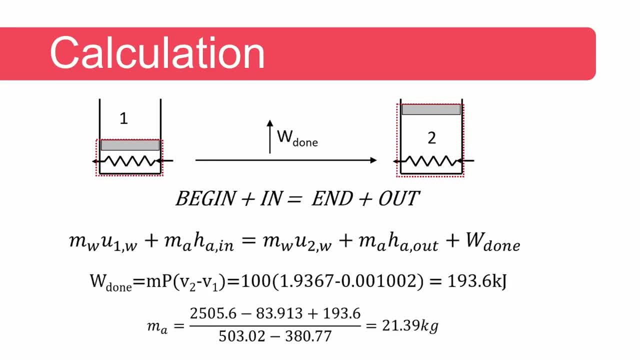 to determine the boundary work. We can read the values of the specific volume of the water and superheated steam from the tables and calculate the amount of air, which comes to 21.39 kilograms. Now we can also approach this problem a bit differently If you draw our system boundaries. 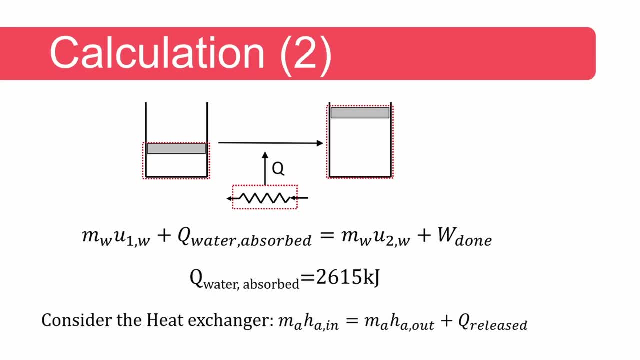 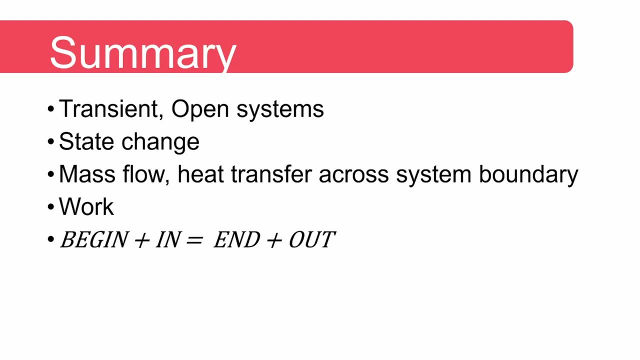 differently. different equations result, but the amount of air will remain the same. See if you get the same value using the two different approaches. So in summary, we consider transient open systems. The state of the system changes from state one to state two and the mass flow and heat transfer can take place across the system boundary. The volume 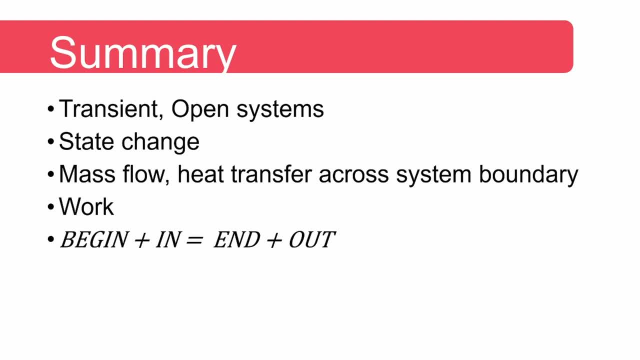 of the system can change, resulting in boundary work, and the conservation of mass means that the mass in the beginning plus the mass flowing into the system must equal the mass in the system at the end of the process, plus the mass flowing out of the system. This is also true for energy. Thank, 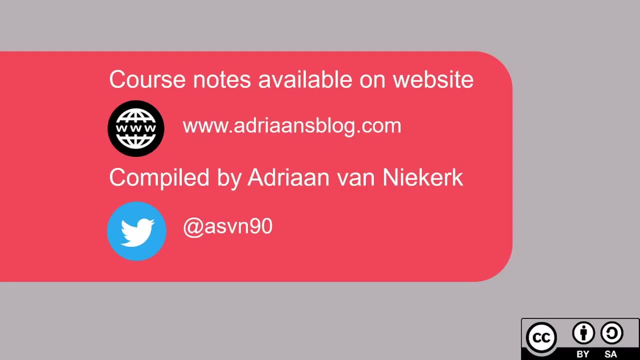 you very much for watching. The last notes which these videos are based on is available on my website, audionsblockcom. I'm also on Twitter. if you want to connect with me and ask any questions there, you're more than welcome to do so. See you in the next video. Bye.